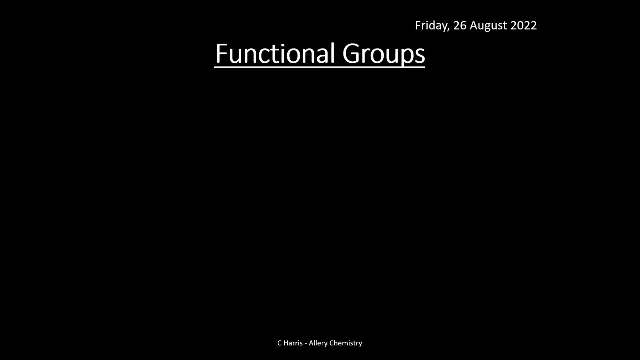 reactions- Not all of them will be on here. It's really difficult to put everything on here, but the vast majority of them will be on here that you'll need to be aware of. Also, what I'm going to do is to summarize the functional groups and types of reaction on this. So this is basically. 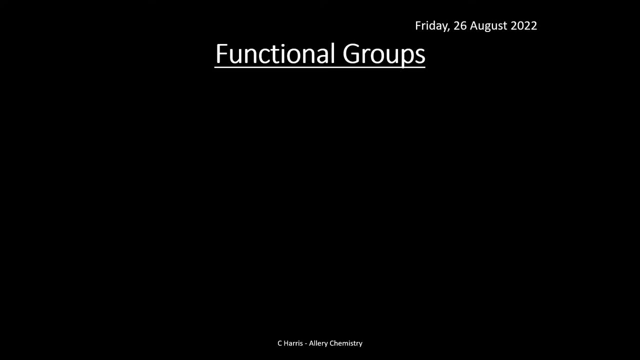 going to summarize all of the organic stuff, because this is the last kind of proper organic topic for year one anyway. So it's a good. it's a nice little summary video, So just to kind of recap. then we need to know various range of functional groups. So alkanes, remember alkanes. 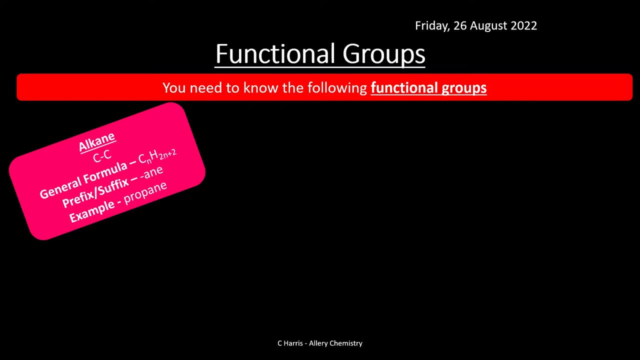 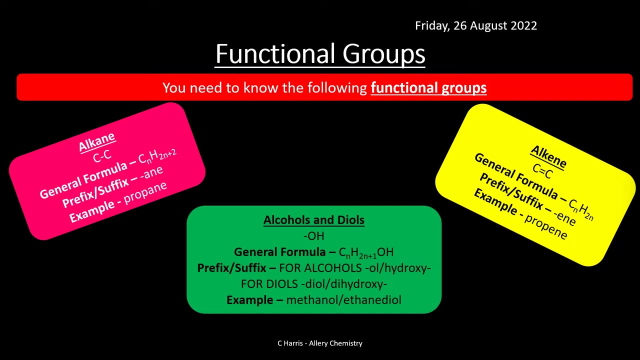 at the end. general formula: CNH2N plus two Alkenes, you will have seen. So these are CNH2N with a suffix of ene, Alcohols and diols. So these have the OH formula, remember. So they normally. 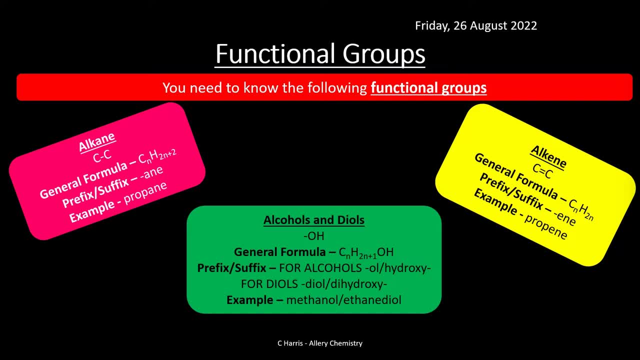 end in al, or sometimes it'll be hydroxy, as you will have seen before. And what I would say as well, make sure that you've gone through all of the organic chemistry topics first- So that's to 20- before you look at this video. I should have said that right at the start, because obviously 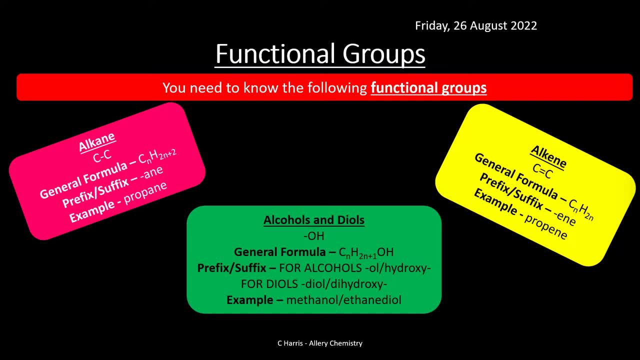 a lot of this stuff is if this is the first time you've seen organic chemistry and you look at this and you're thinking what on earth is he talking about? So make sure you're familiar with the kind of fundamentals of organic chemistry. This purely summarizes it all. But anyway, if you have seen 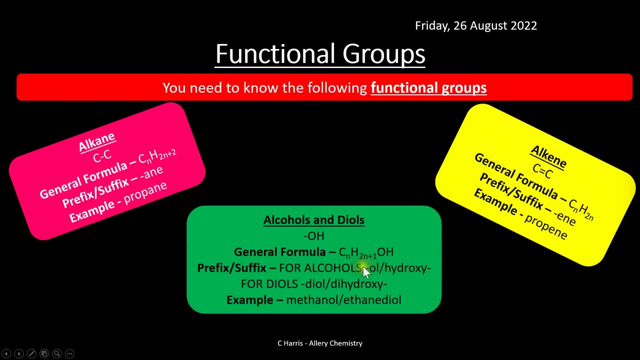 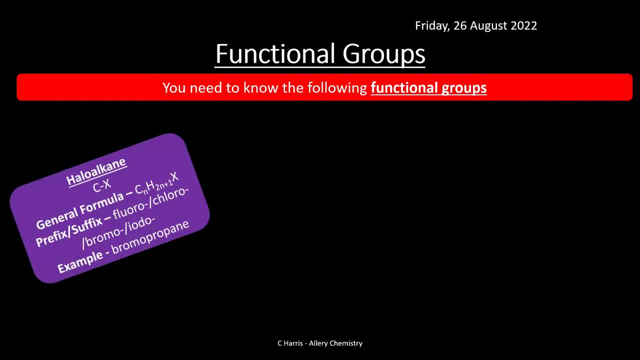 the other videos, then you would notice that there is hydroxy and alcohols as well, Or the end in alkenes, or halogen or alkenes. they're also known as RCX. So these are basically your halogens. 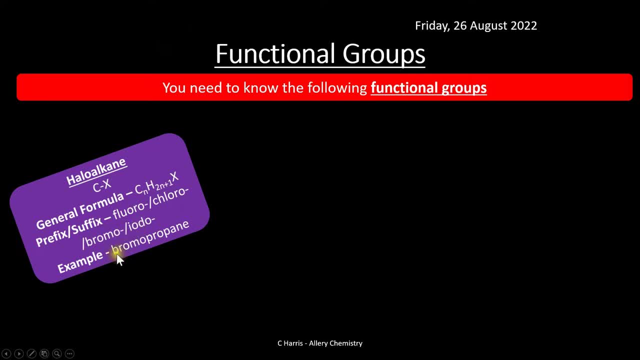 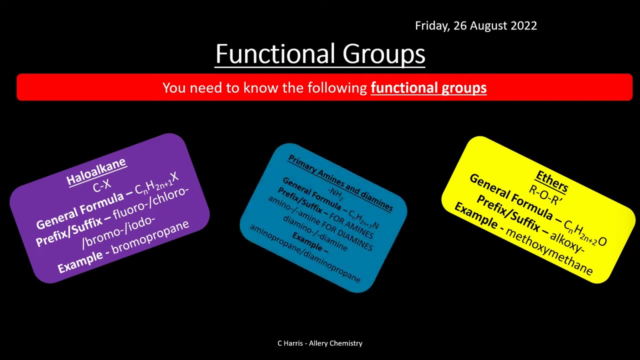 So there'll be fluoro, chloro, bromo and iodo. So, for example, bromopropane is an example. Ethers- you might have seen a few ethers. You won't see many of these, to be honest, but they have alkoxy in the middle, So that's the name of an ether. 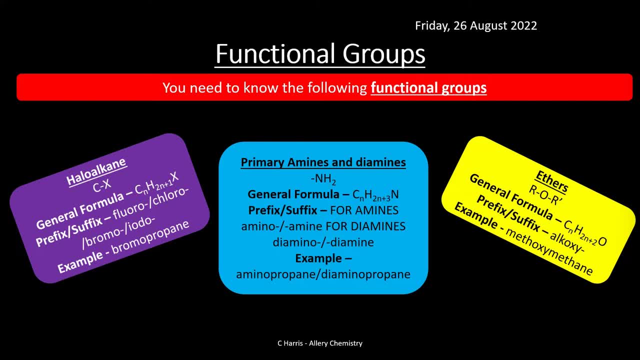 Primary amines and diamines. you would have seen this in the nitrogen compounds topic. So this is 19,. topic 19. And you would have seen it in the halogens group 17 topic as well. So general formula: CNH2N plus 3N, So they always end in NH2.. Now, that's obviously for amines. 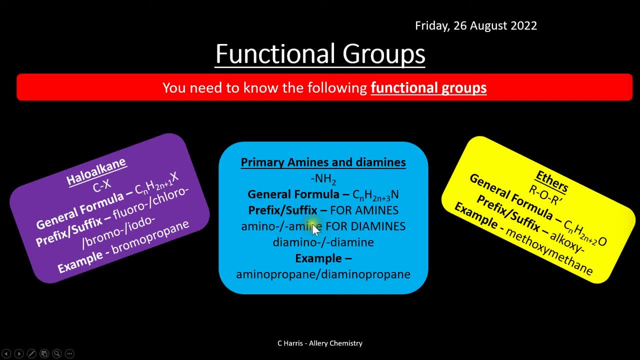 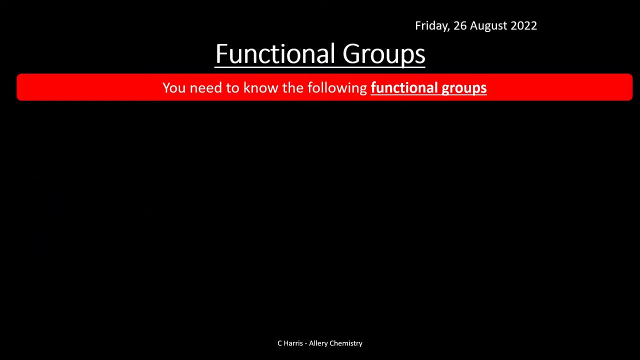 We either use amino or end it in amine- You're mainly going to see this, to be honest- amines, And for diamines you end it in diamine. So that's just some examples there. Okay, aldehydes, These have the C-1.. 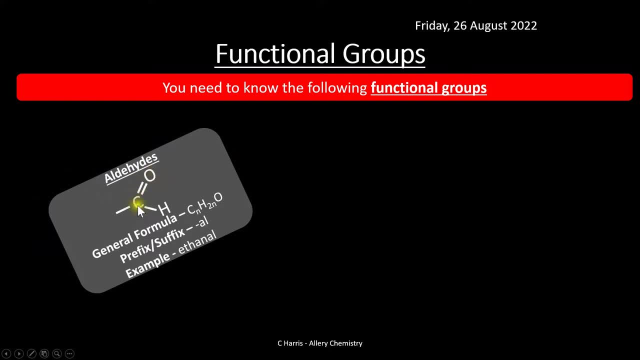 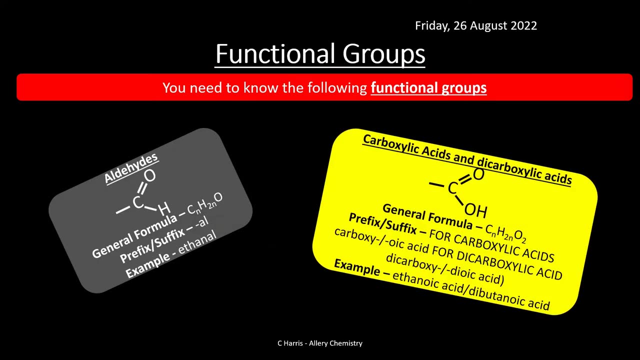 C double bond, O group on the end. So these are always at the end of a carbon, remember, And they end in L, a bit like ethanol. And then obviously you've got carboxylic acids and dicarboxylic acids. 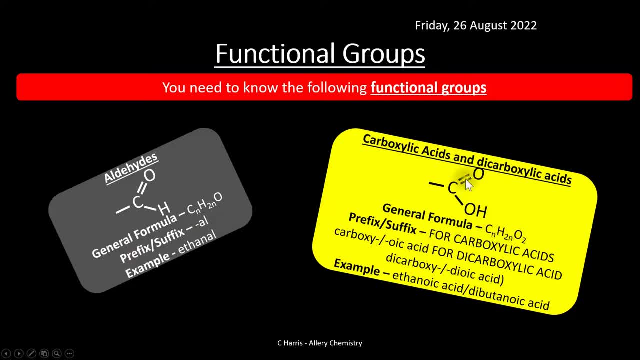 So that's CNH2NO2.. So this has C double bond, O or H. Remember that's a carboxylic acid, So they end in Oic acid at the end. That's really the types you're going to see. 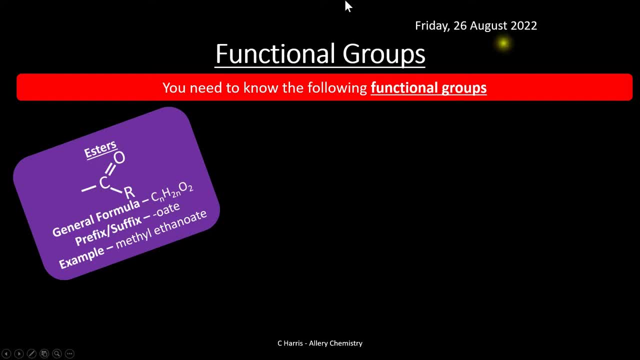 Esters. Obviously, these are derivatives of carboxylic, So these have double bond R And these end in O8. So, for example, methyl ethanoate, depending on, obviously, what's actually bonded on there. So make sure you wear esters. 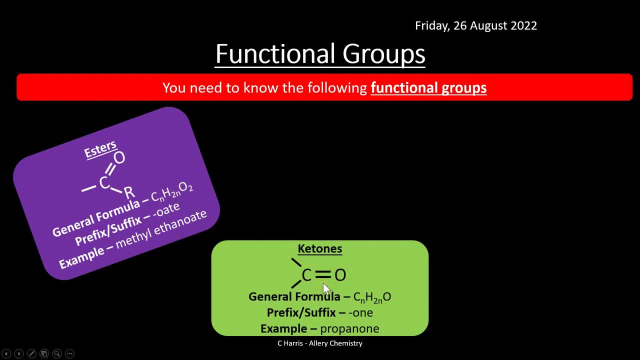 Ketones. Obviously these are a bit like aldehydes, but the carbonyl group here, the C double bond, O, is in between two other carbons And they end in O, for example propanone Nitriles. So these have got CN. 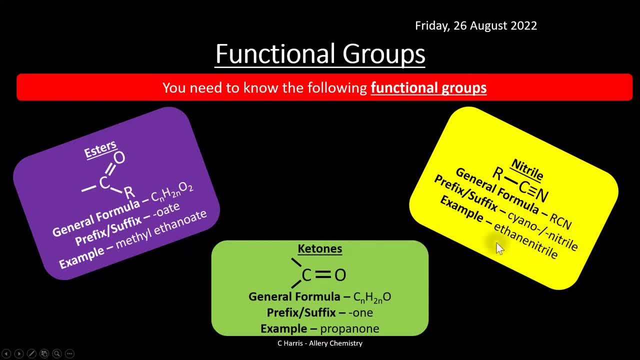 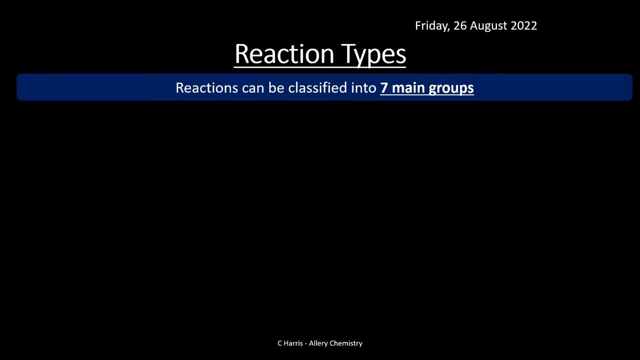 At the end of them. So, for example, they'll be nitrile at the end. For example, ethane nitrile is a good example of that. OK, you also need to know some reaction types as well, And we've got seven main types of reactions. 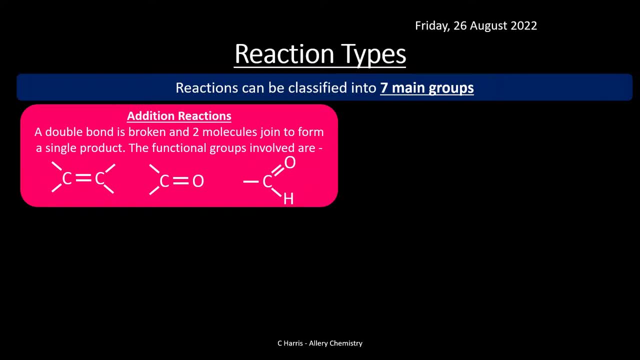 Again, you will have seen these already throughout all the other organic topics. This is kind of summarizing them. So you've got addition reactions And remember. this is when you add across a double bond and two molecules join to form a single product. 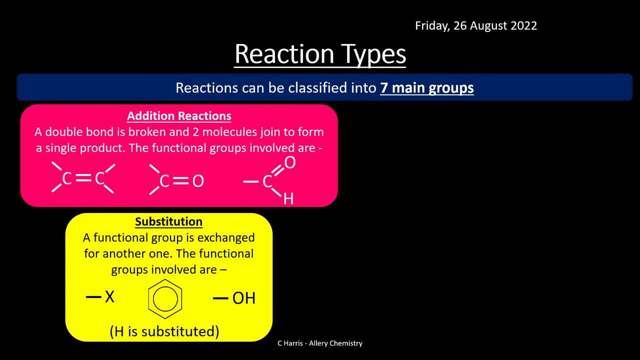 You've got substitution reactions. So this is where you're swapping one functional group for another or one atom for another. So you've got various examples there of halogen, So halidine- sorry halogen- or alkane. It might be an alcohol, benzene you'll see in year two, but you'll kind of come across that later. 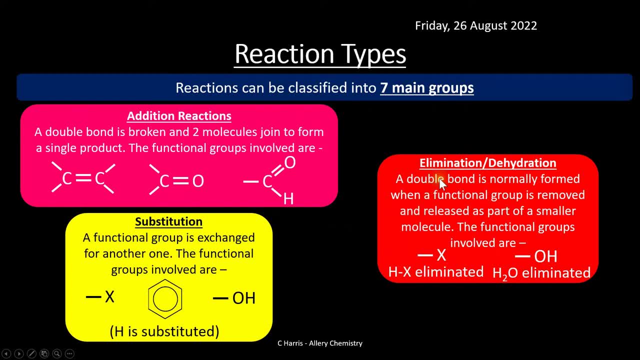 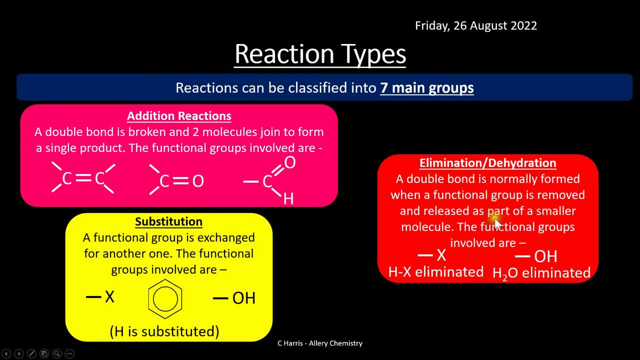 You've got to form an alkene as well. So if you're eliminating, you'll form an alkene, So something with a double bond, So for example, X. if you're removing a halogen, it might be HX that's being eliminated. 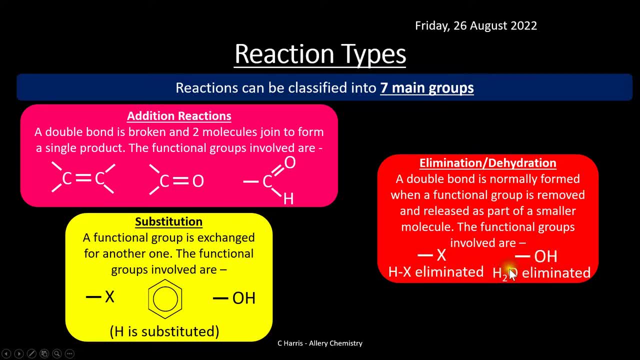 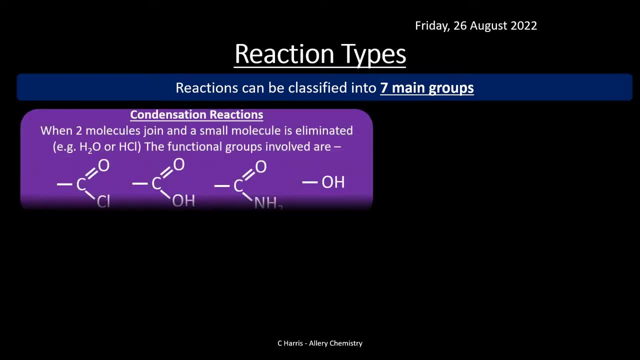 Or if you're removing an OH, say, from an alcohol, then you're eliminating water And that's why they call it dehydration reaction as well. So they've got kind of two names Okay. condensation reactions are when you kind of emit a water molecule, or it could be HCL. 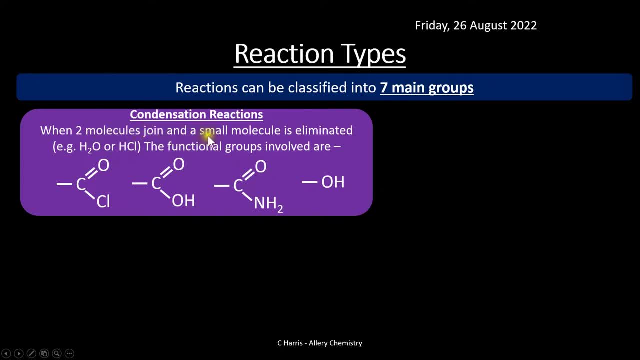 It could be either of them. So this is when you get two molecules joining and the smaller molecule is emitted from or eliminated from the actual reaction. So functional groups generally involved with these reactions are acid chlorides, which you'll see in year two. 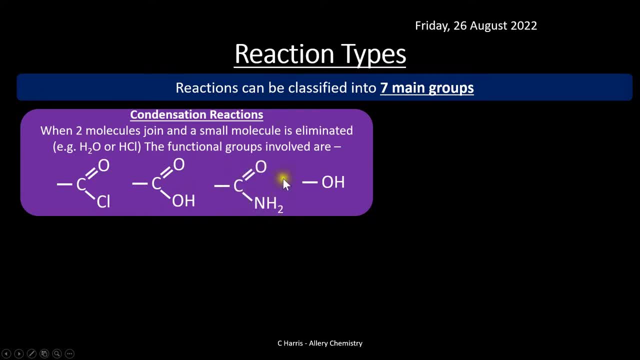 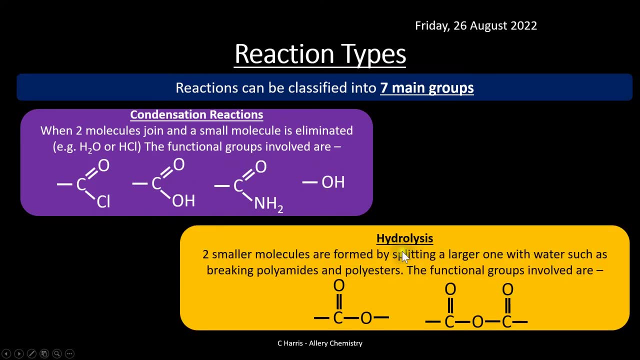 carboxylic acids, amides, which again you'll see in year two, and OHs, so alcohols, which obviously you've seen already. Hydrolysis: hydro meaning water, lysis meaning to split, So this is splitting of a molecule using water. 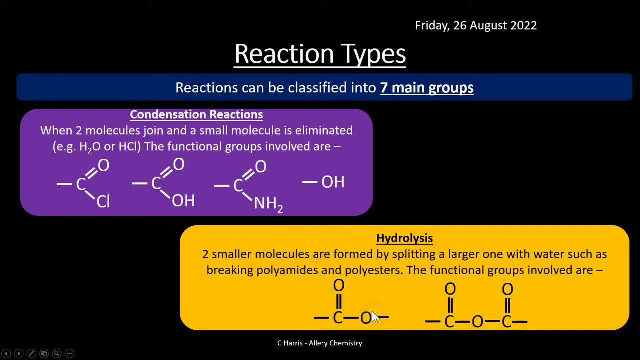 So obviously you're forming two smaller molecules. This could be, for example, breaking polymers apart. It could be esters, for example. So I know we've got polyesters, but you can break esters apart, as you've seen previously. 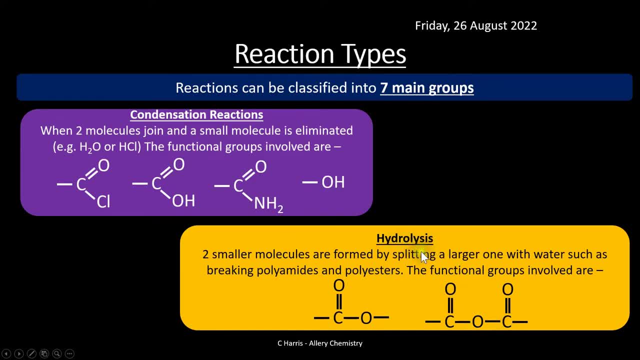 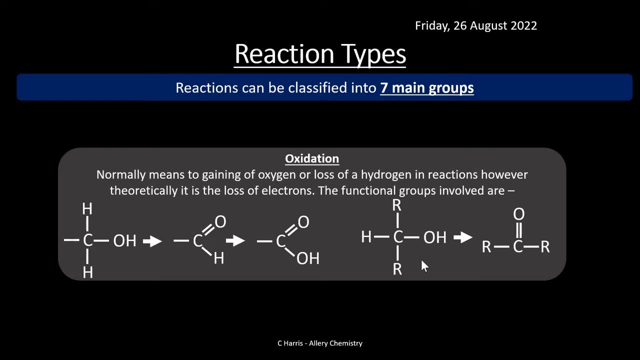 So this is just breaking any molecule with water. And finally, is oxidation. So no, it's not. It's not finding, it's penultimately, because you've got reduction after this as well. So oxidation is basically, you're reacting a molecule with an oxidizing agent to form a different product. 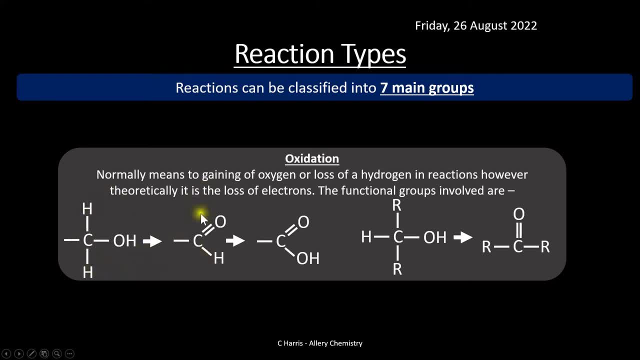 So classic example here would be primary alcohol to aldehyde, to carboxylic acid, or secondary alcohol to ketone. So that's a classic sign of an oxidation reaction And then obviously reduction is just going backwards. So this is carboxylic acid. 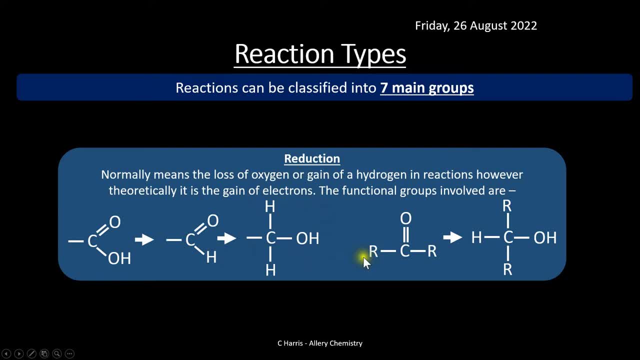 Form: an aldehyde to a primary alcohol and then a ketone to a secondary alcohol, which is obviously at the end there. So they're kind of like your main types of reactions there. Now, what we have to do is then kind of put all this together. 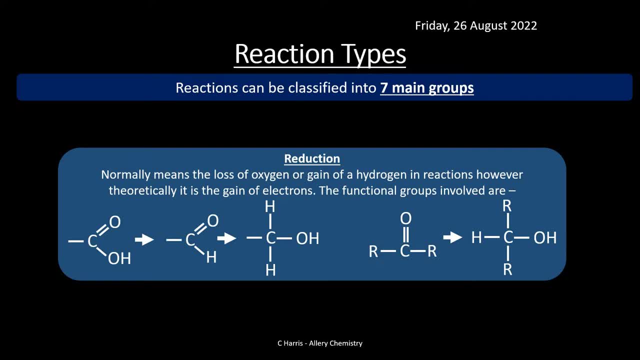 And you've seen an awful lot of reactions, to be fair for organic chemistry. So what's nice is to try and kind of put all this together, show you kind of how each of these chemicals kind of interact and show you multiple steps of how you make them. 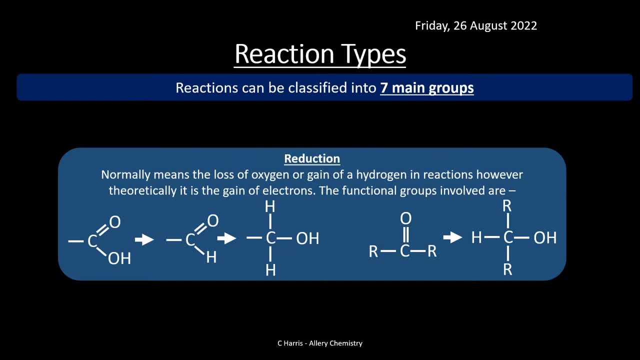 Now what the example do we expect you to know is the reaction conditions of some of these reactions and what forms what. This can take a lot of time, And the best thing to do with anything like this is to do it over time. Never just sit down and try and remember all of these in an hour or so, because it isn't going to happen. 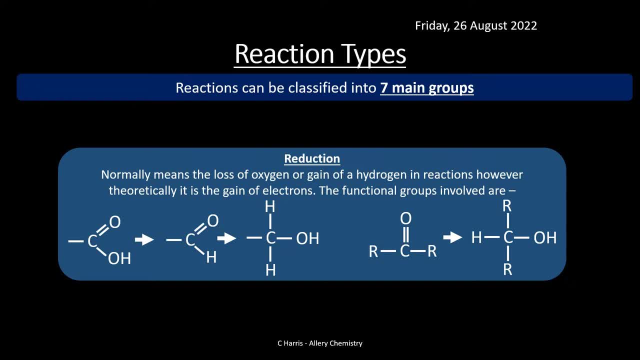 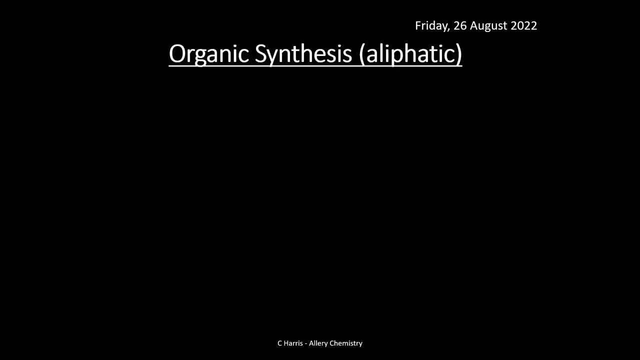 You've got to make sure that you're kind of remembering these reactions just over time, over weeks and months, as you're studying, and you'll pick these up. But this next slide is just really for a summary Of the reactions that you will have seen during your time in year one, chemistry. 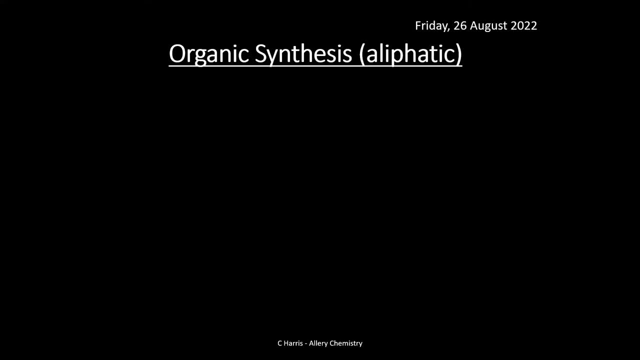 So these are all what we call aliphatic. All that means is just straight train hydrocarbons or straight chain based. So they don't well, not straight chain, but they don't have a benzene in there. Basically, when you do year two chemistry, if you do do that, then you will be introduced to what we call aromatics, which basically they have a benzene ring in there. 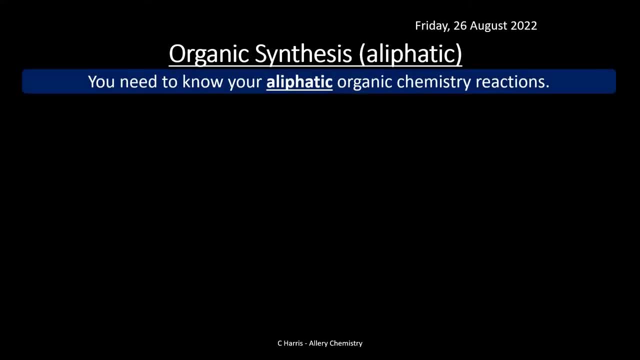 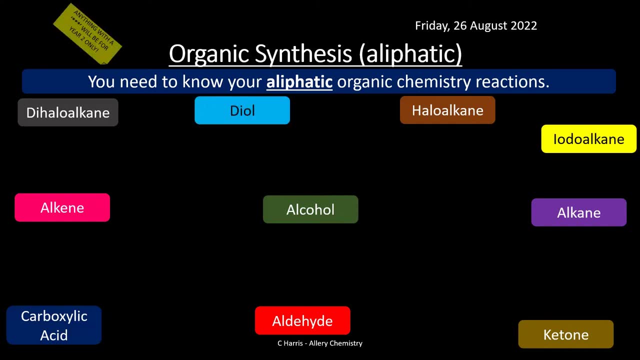 But for this purpose. obviously, you don't do anything to do with that in year one, So You need to know these reactions. Now, what I'm going to do is I'm going to put some of these up on here. So these are some of the ones that that you'll be familiar with. 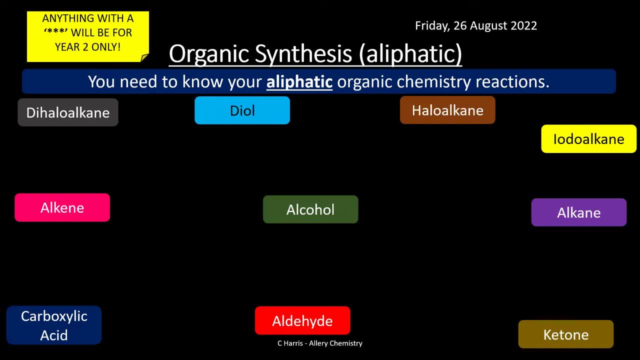 Anything with a triple star will only be for year two. But all of these you should be able to. you should know effectively And what I'm going to do. I'm going to do this differently, So what's going to pop up in here is an arrow. 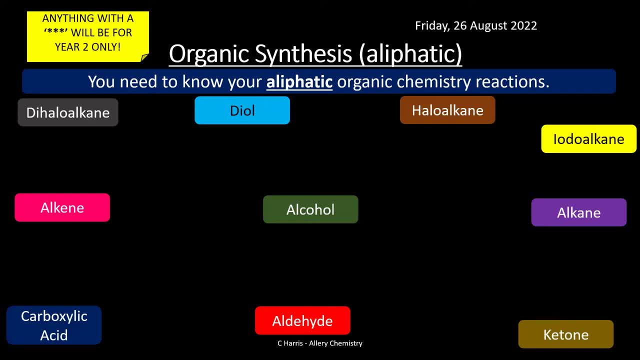 And I'm going to. you can pause the video when the arrow comes up. Try and see if you can work out what the reaction conditions are And then unpause the video and then see if you are right. So this is a good way of kind of summarizing this. 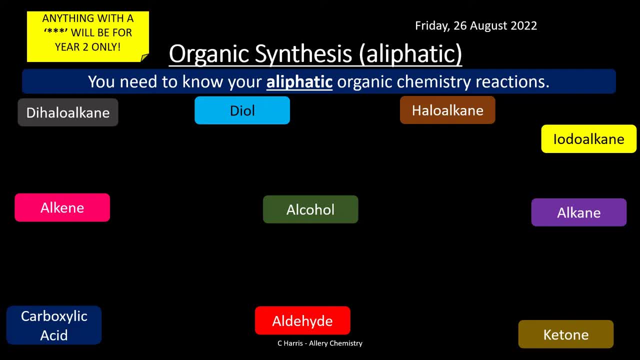 I think that's probably a better use of this. Otherwise, I'm just going to be going through a series of reactions. So let's do the first one. So let's say we're going from alcohol to aldehyde. So if you want to pause the video now and then see if you can write down your reaction conditions, 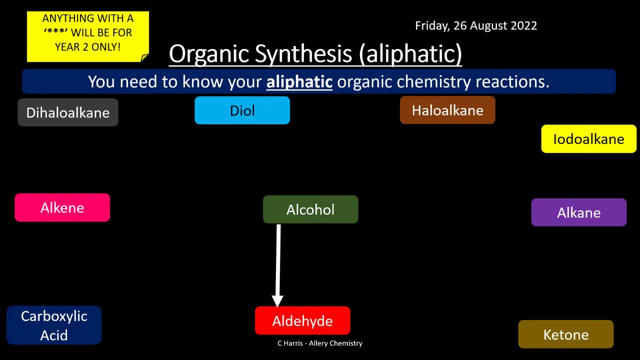 And then obviously I'll reveal the answer. So I'll do it for all of these. So obviously this one is going to be potassium dichromate and sulfuric acid Eaten with a primary alcohol. That's what the one, the one little degree, that's primary. 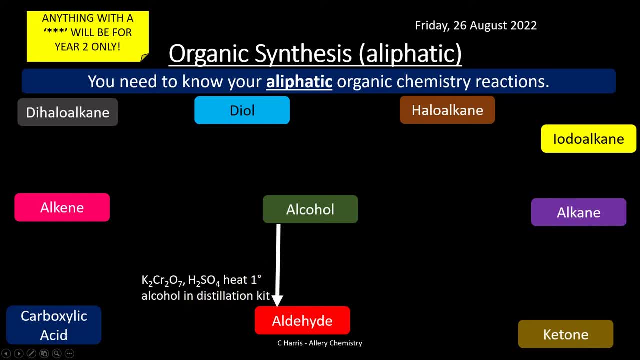 Primary alcohol in distillation kit: Okay, so let's go backwards. Aldehyde to alcohol- Okay so, this one's sodium borohydride in methanol and water. So let's do aldehyde to carboxylic acid- Okay so this one is potassium dichromate, sulfuric acid, catalyst and reflux. 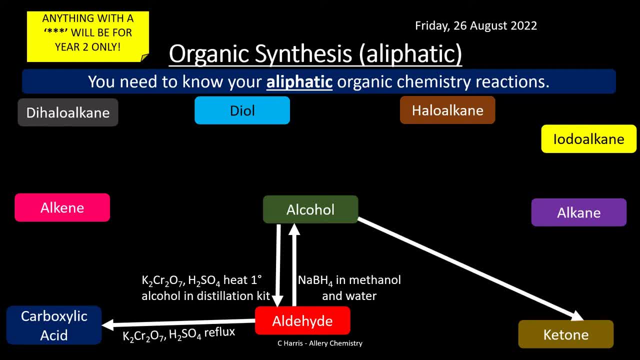 So what about alcohol to ketone? Okay, so this one's going to be potassium dichromate, sulfuric acid and some heat, And it's a secondary alcohol for this one Obviously forming a ketone. What about ketone to alcohol? 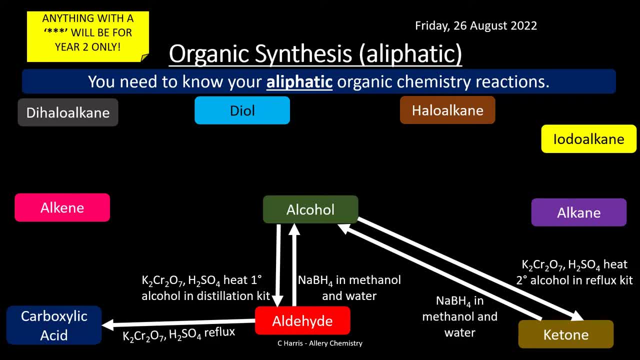 Well, this one's going to be sodium borohydride, So it's a reducing agent in methanol and water. So what about alcohol to alkene? Well, this one's going to be concentrate sulfuric acid, or you can use phosphoric acid and some heat. 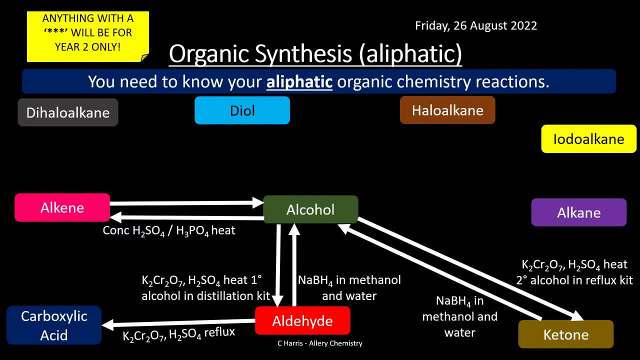 So what about going backwards? Alkene to alcohol? Okay, well, this one's going to be steam, some phosphoric acid catalyst, 60 atmospheres of pressure and 300 degrees Celsius. Okay, so what about alcohol to haloalkane or halogenoalkane? 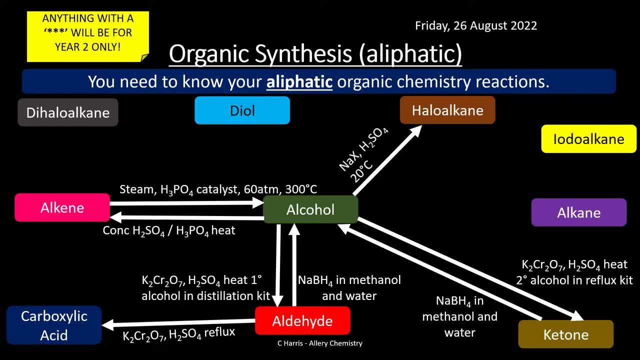 Okay, well, this one's going to be sulfuric acid, Sodium halide, so NAX plus H2SO4 and 20 degrees Celsius. So what about going backwards? Haloalkane to alcohol? Okay, well, this one's going to be warm sodium hydroxide, some water and it's all done under reflux as well. 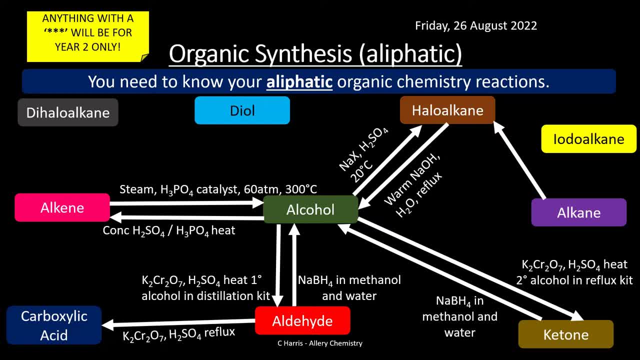 What about alkane to haloalkane? Okay, well, this one is the radical reaction, So this is using UV light And obviously you use a halogenoalkane, So you use a halogen X2 for this. So what about alkene to haloalkane? 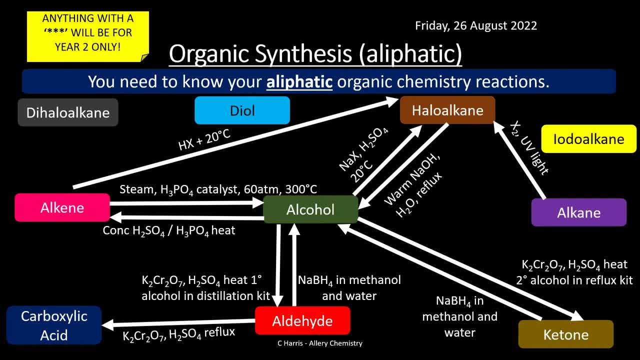 Okay, so this one's going to be HX, so it's your hydrogen halide, and it's done at 20 degrees Celsius, So it's just a different temperature. Okay, so what about haloalkane to alkene? Okay, so this one's going to be potassium hydroxide ethanol, and it's going to be done under reflux. 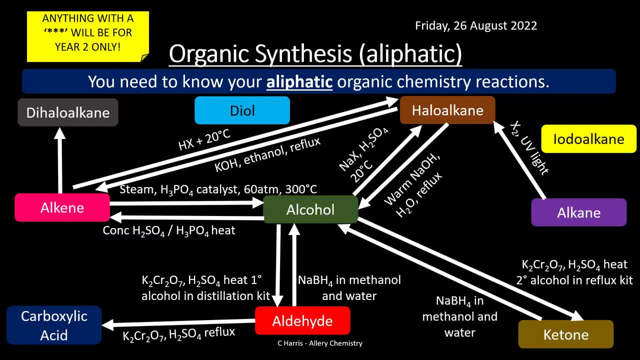 What about alkene? What about alkene to dihaloalkane? Okay, so with this one, you're going to use your halogen and it's going to be 20 degrees Celsius, So this is basically adding bromine to your alkene. 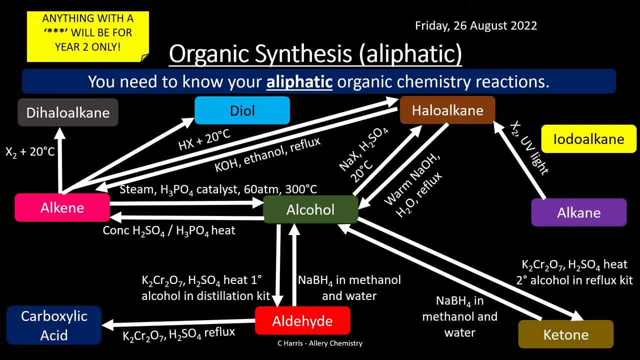 It's a decolourisation of bromine, remember? Okay, what about alkene to diol? Okay, well, this one's going to be acidified potassium manganate solution, and this is going to be done at 20 degrees Celsius. 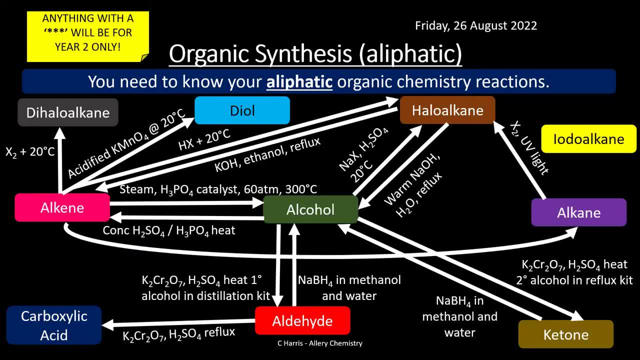 And what about alkene to alkane? Okay, well, this one's going to be hydrogen and it's going to be a nickel catalyst and it's going to be done at 150 degrees Celsius. And what about alcohol to iodoalkane? 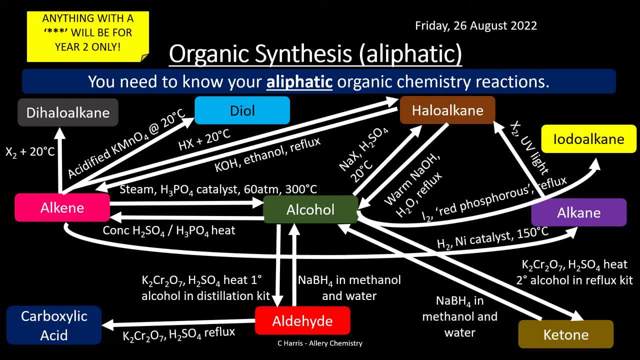 Okay, well, this one's going to be iodine, and this is your red phosphorus and reflux as well. So remember that kind of- it's a very specific reaction for that one. And what about carboxylic acids to alcohol? Well, that one's going to be lithium, aluminium hydride. 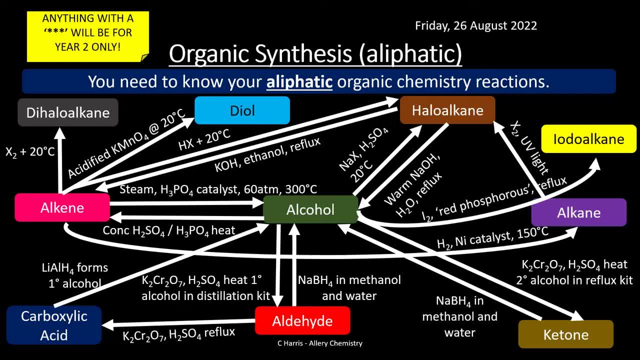 It's your reducing agent and that forms a primary alcohol as a result. Okay, so that's the first slide. There's more reactions to come. As you can see, there's a lot on there, a lot of different reactions. So you can see why you should be doing this over time really. 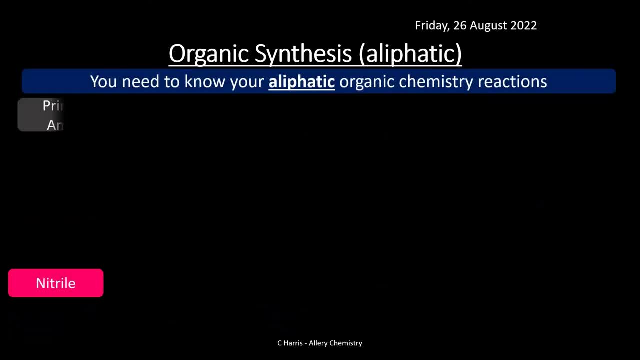 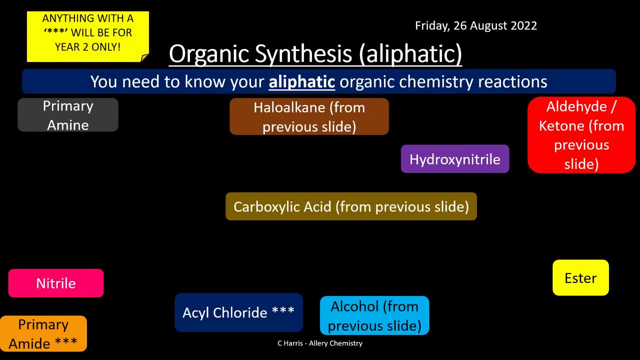 Right, I'm going to clear the board And I'm going to bring up a load of new ones here Now, like I say, the ones which have been dragged from the previous slide. I've put from previous slide, as you can see, obviously. 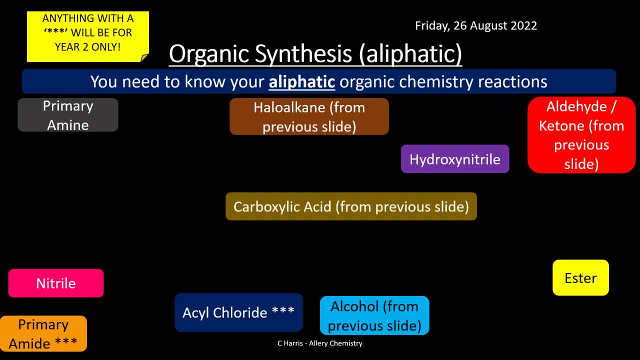 Anything with three stars you don't need to do So. I'm just going to kind of. they're still going to pop up on the screen, but I'm just going to skip past them because you won't need to know them until year two. 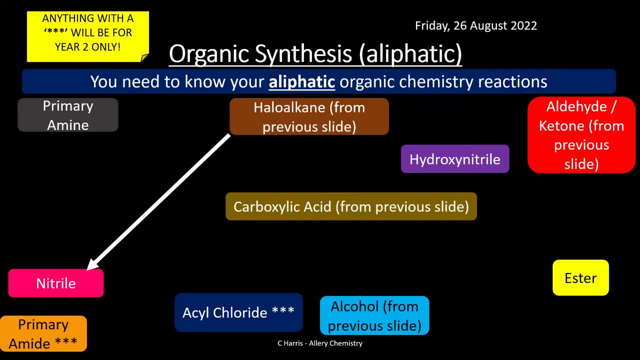 Okay, same again. So let's do haloalkane to nitrile. Okay, so this is going to be potassium, cyanide and ethanol and reflux. So what about nitrile to primary amine? Okay, well, this one's going to be lithium aluminium hydride. 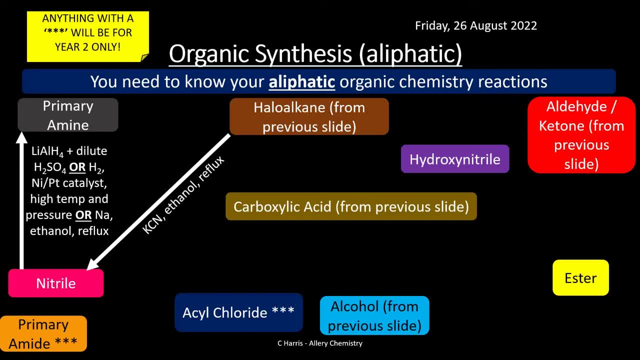 and we're going to use dilute sulfuric acid. or we can use hydrogen with a nickel platinum catalyst, high temperature and pressure, or we can use sodium, ethanol and reflux. So any one of them will deliver the results to, or from nitrile to primary amine. 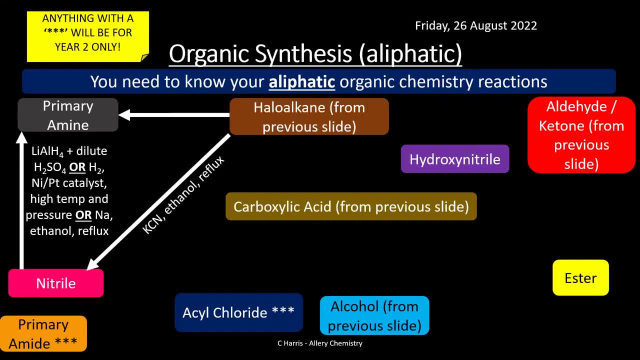 Okay, so what about haloalkane to primary amine? Okay, well, this one will be ammonia and heat. And so what about nitrile to carboxylic acid? Okay, well, this one's going to be dilute hydrochloric acid. 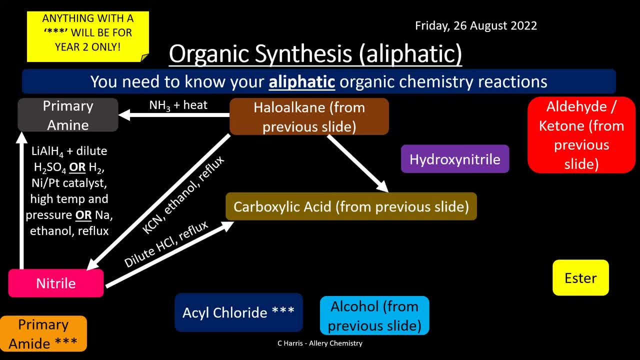 so dilute HCL and reflux. What about haloalkane to carboxylic acid? Okay, well, this one's going to be magnesium. magnesium and a dry ether and carbon dioxide in dilute acid. So that's obviously going from there. 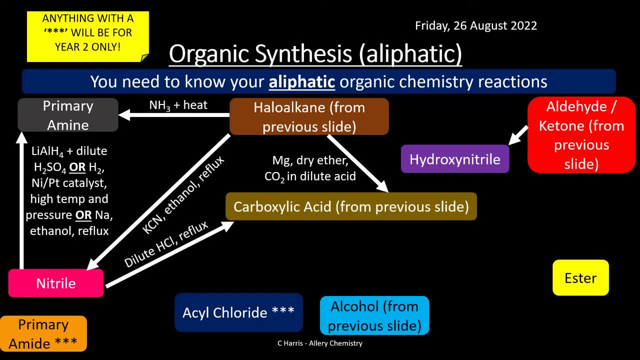 What about aldehyde or ketone to form hydroxynitrile? Okay, well, this one's going to be potassium, cyanide, sulfuric acid, and it's all done at 20 degrees Celsius. Okay, isylchloride to carboxylic acid. that's the reaction there. 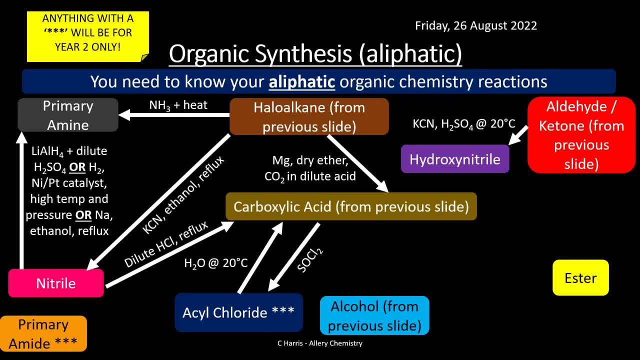 Again, you'll kind of come on to this in year two, And obviously vice versa, Okay, so don't worry too much about that. in year one: Okay, aldehyde and ketone to an ester. Okay, well, this is going to be concentrated sulfuric acid. 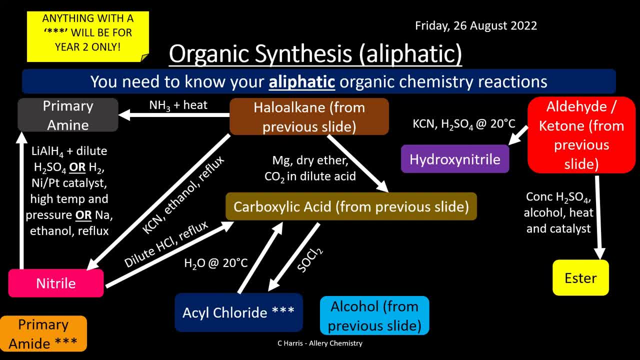 alcohol, heat and a catalyst. I'm just going to use a catalyst for that. So this is sulfuric acid catalyst Ester to carboxylic acid. Okay, so this is your hydrolysis reaction. Okay, so this is your hydrolysis reaction.